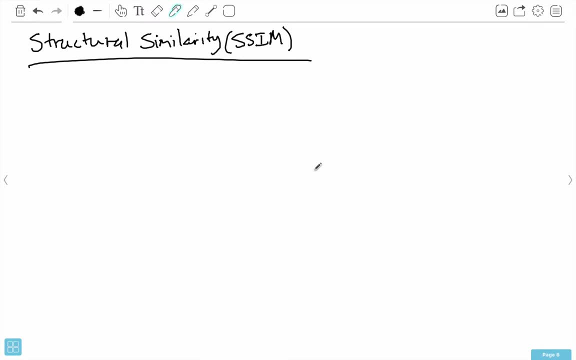 You know, when humans look at images more holistically, structural similarity tries to capture this using statistics, And that's the issue with mean squared error is that we're not looking at, we're just looking at all of the pixels, And as humans, we don't do that. 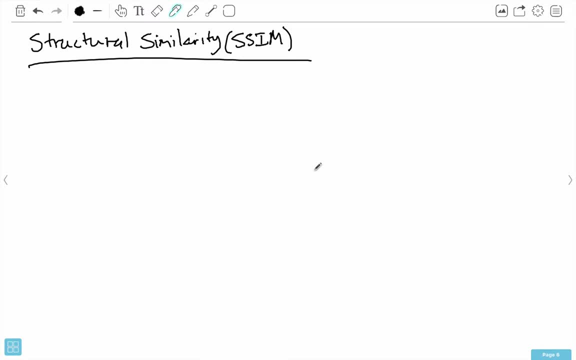 You know we can't see all of the small variations and noises in our image And you know, overall it doesn't really matter if there's a little bit of. you know, if we're a couple, if we show you two images and one of the images has all the pixels that are just shifted by like one value. 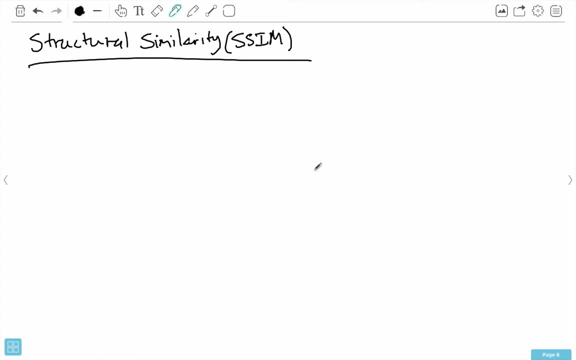 then you're probably not going to see, You're probably not going to notice the difference at all And you'll say, well, these two images are exactly the same. But mean squared error will see, and it will pick that, pick that up, you know. 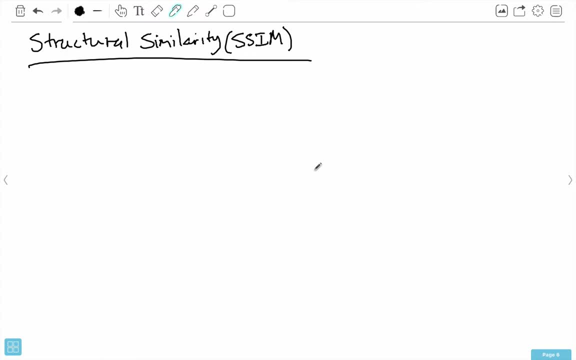 So, instead of doing these pixel-wise independently or treating a pixel independently, structural similarity actually looks at groups of pixels to try to better determine if two images are different or not. And so let me- Let me actually write this down- that MSE- and also some squared error, if you choose to use that- you know they look at pixels individually. 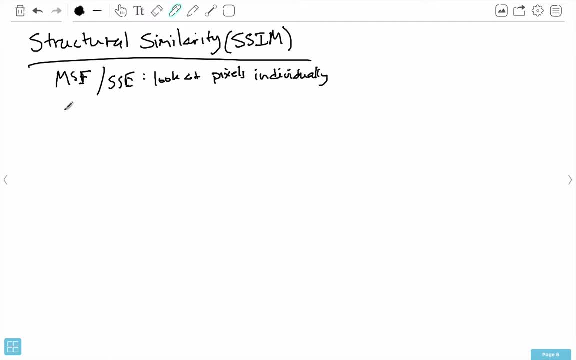 Look at pixels individually, Right, But with structural similarity that's a terrible. Structural similar Third time's a charm With There we go, The structural similarity. We look at groups of pixels, So groups of pixels. And this is a bit better than looking at pixels individually, because then all those small changes of noise and variation, you know, don't tend to affect groups of pixels than they do with individual pixels. 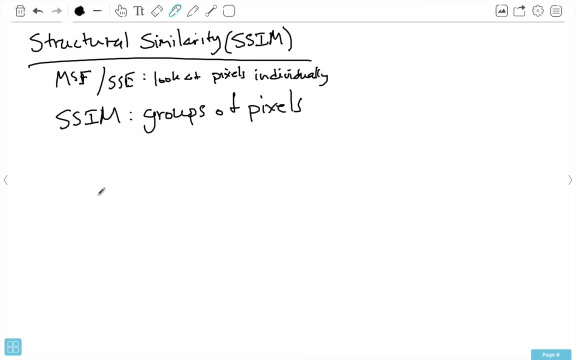 Right, And as it turns out that some structural similarity is actually a, actually a product of three other kinds of measures, So let me actually write out structural similarity. So structural similarity between an A and a B is actually a product of some other things. 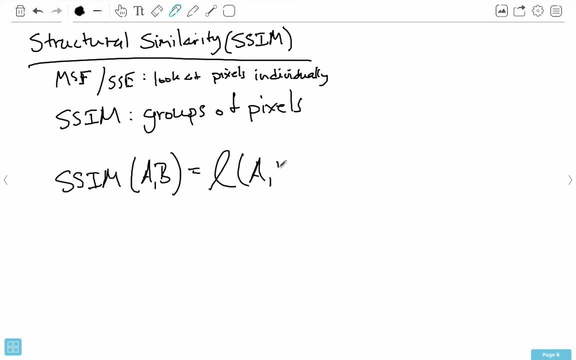 It is a product of L of AB, times Times, C of AB, times S of AB. I'm going to explain what these are in just a second. So L is stands for luminance, So luminance, C is contrast And S is structure. 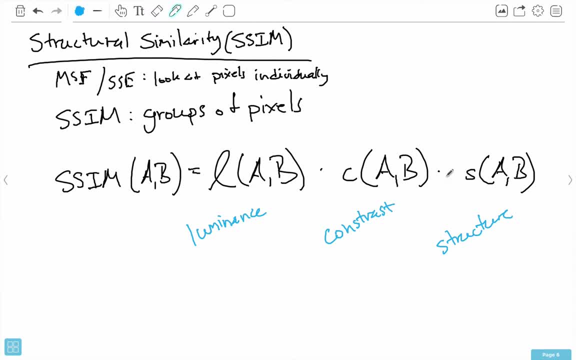 Okay, And I'm not actually going to expand this out, Because there's an actual, you know formula dealing with Individual, you know pixels and actually, or actually with groups of pixels, using statistics like the mean and variance, And I actually don't want to expand that out because that kind of gets more into statistics and histograms and stuff that I don't really want to get into that much. 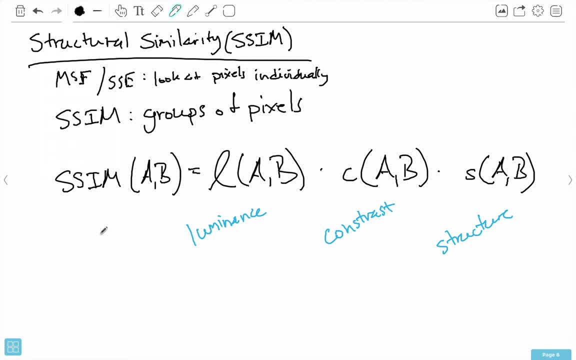 It requires a pretty decent amount of knowledge about statistics, But A and B turns. it turns out that When you look at groups of pixels, then you get a better representation of the image and a better representation subsequently of the difference between images when you look at groups instead of just an individual pixel. 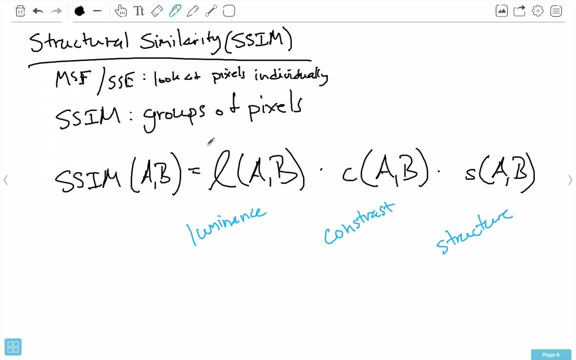 And so you know, we look at things like we look at the histogram, basically, we look at the averages of pixels, we look at the spread of a group of pixels, And all of these measurements use statistics to actually determine similarity. We get a kind of a better idea of the difference between the images when we look at groups instead of just individual pixels. 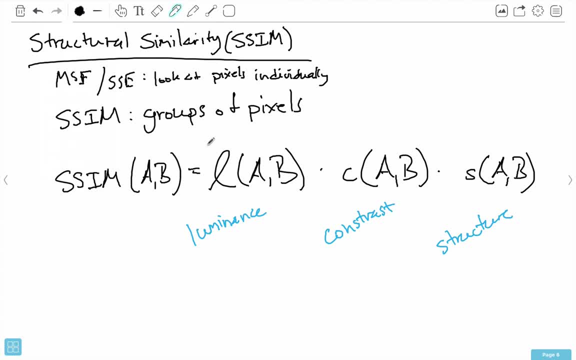 And you know, in the next video I'm actually going to show you why this is a bit better and this is a bit more, slightly more representative of how humans perceive images. And you know, there's more, There's more. 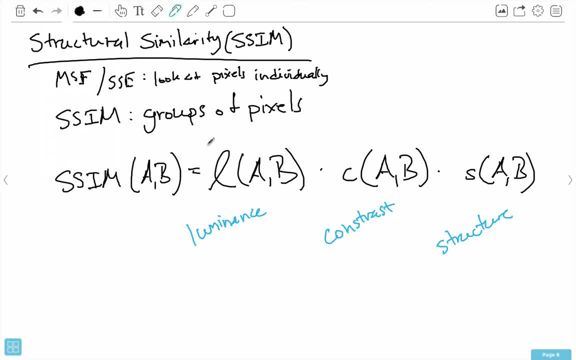 Topics to discuss. uh, about that that we won't be able to get into. but structural similarity is a really good measure of image difference and the good thing about structural similarity- that's much different than mse mean squared error or some squared error- is that it actually has a lower and 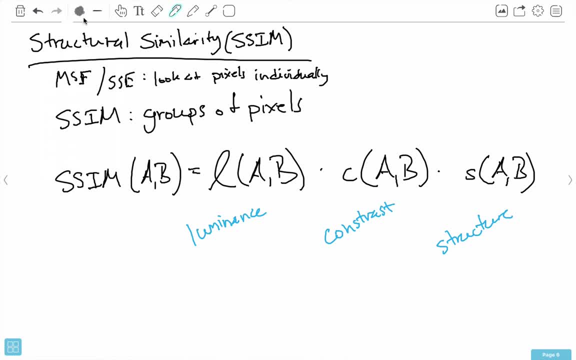 upper bound. so what i mean by that is, let me just use a different color here- is that structural similarity is always between minus one and one, where positive one is perfect match and minus one we're not going to talk too much about. but oops, minus one means that it is imperfect. 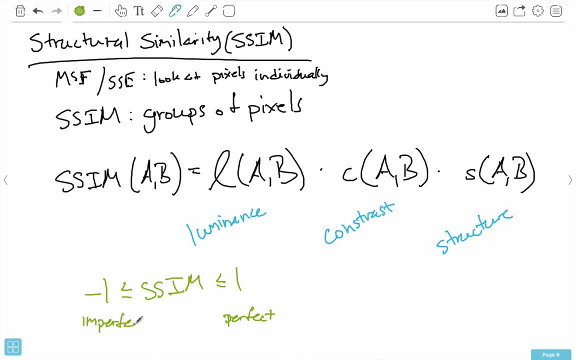 or i should say it is perfectly imperfect and that just has to deal with the way that the stats work out. but we're we just don't consider this, this realm here, we're just more concerned about the scrum, so the closer that the result of structural similarity and returns a 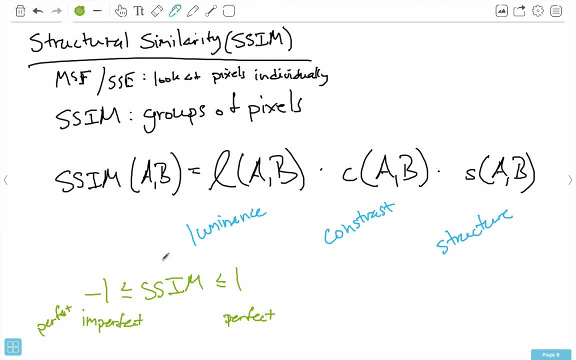 number, just like mean squared error and some squared error closer is to one, the closer two images are to being related, or i should say the closer the two images are to being exactly the same, because if i have a structural similarity index, i get the value back: it's one. then i know. 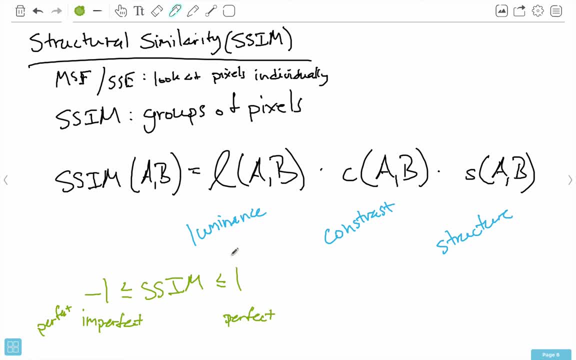 that these two images are exactly the same. if it's a little less than one, then i know that well, they're a little bit different, and so this kind of works in a similar fashion as mean squared error. but, if you notice, mean squared error actually doesn't have. 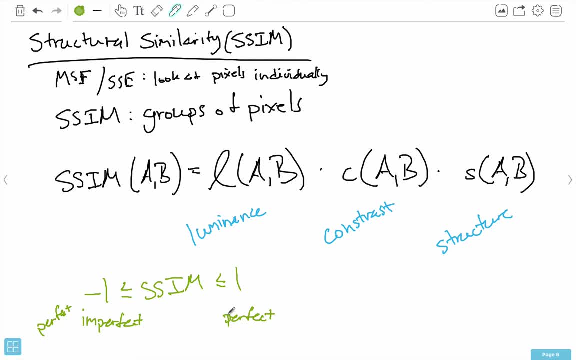 an upper bound. it could, i mean, besides barring any sort of, you know, bounds that you put on the pixel values themselves mean squared error just has a lower bound of at least zero, and then you know, it could be any large number after that, but with structural similarity it's always between. 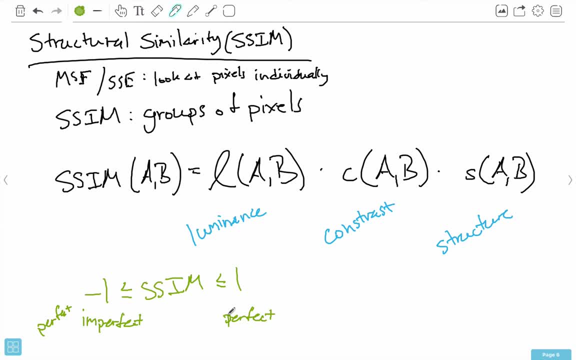 minus one and one, and that's really nice, and so i think this is something that i'm going to stop this video and we're actually going to see an example of structural similarity and how it compares to mean squared error in the next video. and don't worry, we don't. 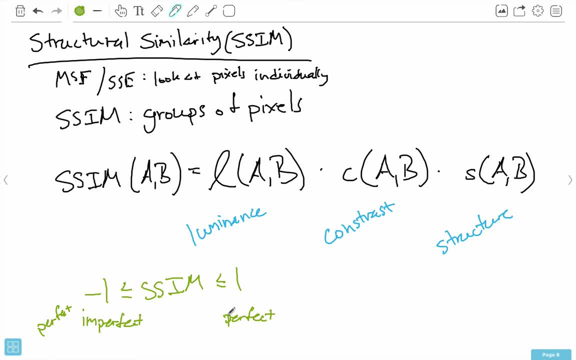 we don't have to implement this at all, like even in, even using numpy, because it turns out there's this library under. so it's a component of sci-fi. it's called a scikit image, or i say it's a component of scikit, not necessarily sci-fi, but 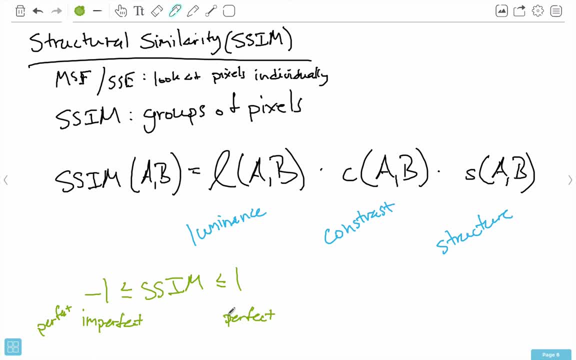 a component of scikit called scikit image and it actually just gives us a function called structural, called ssim, and you just pass it to images and it computes a value. so it's almost, it looks almost exactly like this. you don't feel like and it has other parameters, but we don't.